we have discussed that. that is used for making hollow superpower in size, and blow molding is also used for making of hollow parts X symmetric parts. so if we can, ah, try to differentiate between the two. in rotational molding we will use a very large size mold, so it will be. 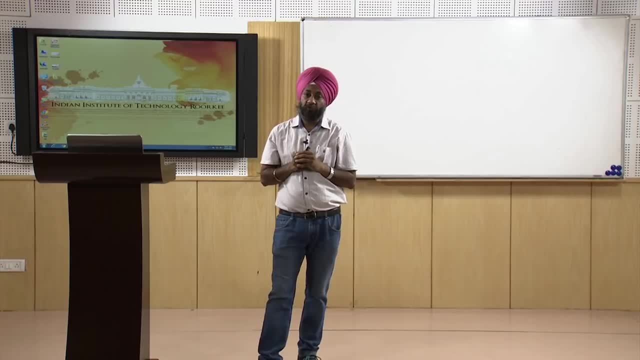 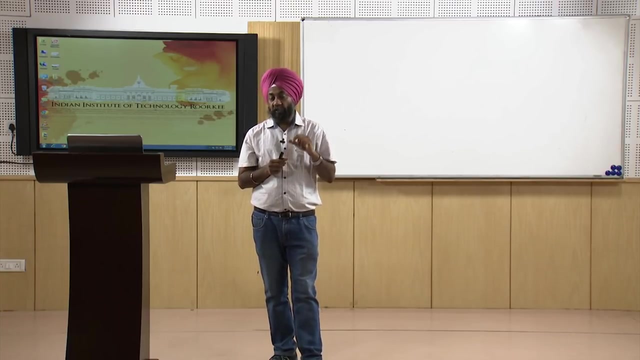 for example, the overhead tanks that we have at our houses, overhead water storage tanks, specifically so they can be made by the rotational moulding process. whereas in case of blow moulding process, our size of the product will be smaller in case of rotational moulding process, if 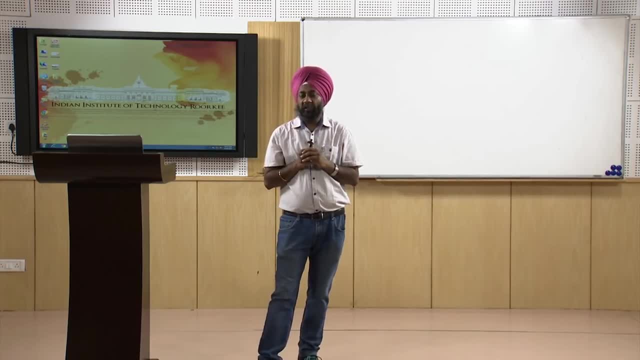 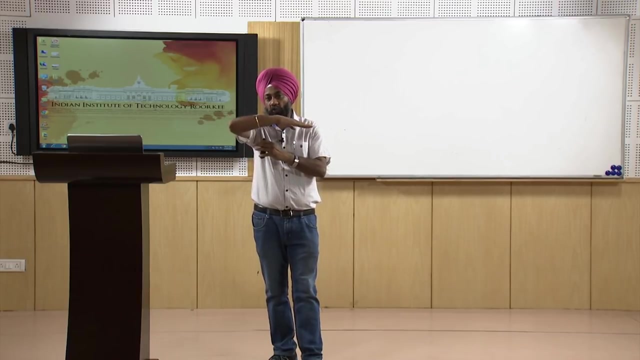 you remember, there was minimum pressure required. the heat or the temperature was more, pressure was less, so we used to input the raw material inside the mould cavity and then we were rotating the mould into principal axis, the, the horizontal axis and the vertical axis. the mould was rotating. 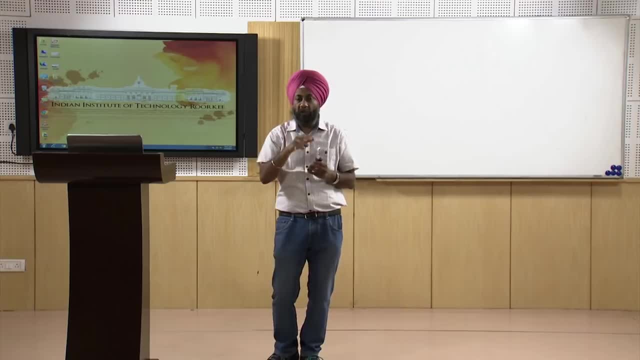 or we were, we were giving a rocking motion to the mould so that the molten plastic inside the mould is well distributed at the inner wall of the mould. and finally, even during the cooling process also, we were giving rotation or or rocking movement to the mould so that the material solidifies inside the mould. and finally, 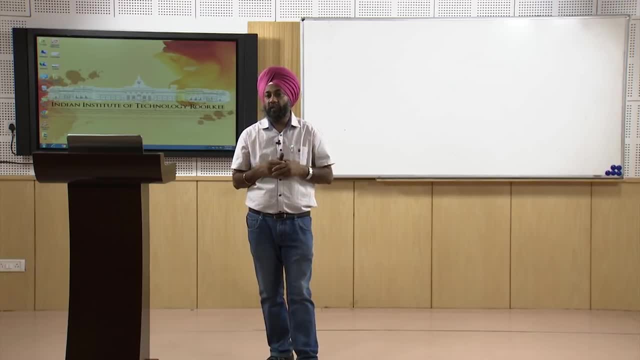 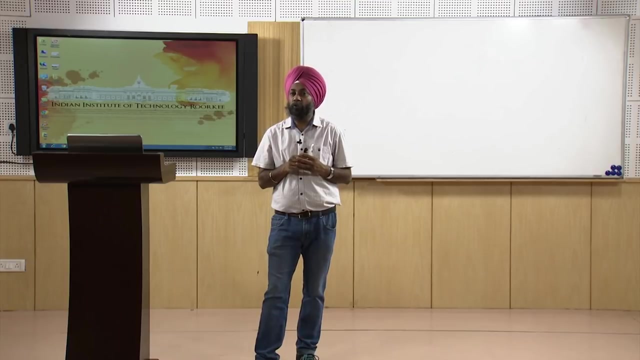 we were opening the split mould and taking out the final product. so that was the basic principle of rotational moulding. so there was no external pressure required. only the rotation of the mould was leading to the distribution or the spread of the molten plastic at the inner walls of the mould, but specifically in blow moulding, as the name suggest, because 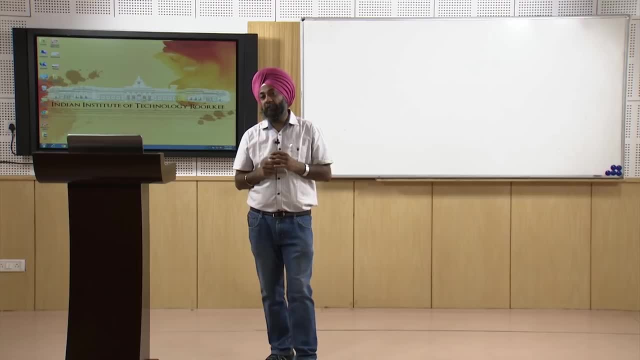 in the mould. fundamental principle, usually the nile moulding is most often used with the你在 the mould due to the inflation of the lieutenantism based on the Hayward analysis of the materialille of the mould and gone. this same procedure is very used in iyi made. 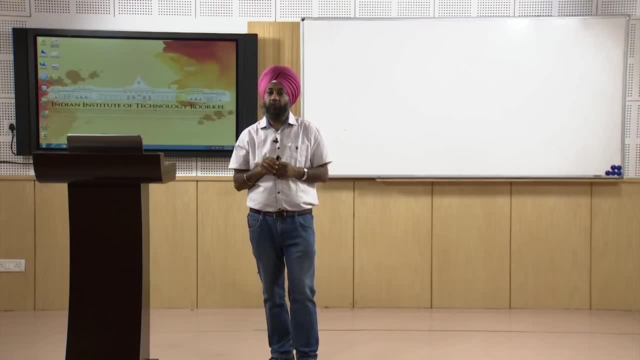 lever, times Wagner's. these processes have been named based on the fundamental principal that is used for forming the plastic. let us take the example of injection molding. why the name injection is coming into picture? because we are injecting the molten plastic through the nozzle into the die. so injection injection can be through a plunger or a ram. 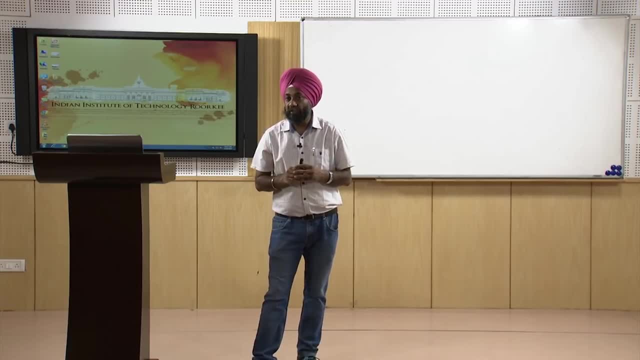 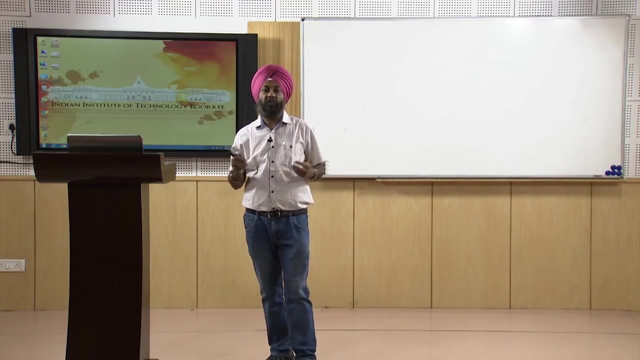 molten plastic is taking place and therefore we name the process as injection molding, rotational molding. the mold is rotating about two principle axis: rotational molding. so from these two examples, let us see why blow molding. and before going to blow molding, let us take another example, that is, transfer molding. in transfer molding, some transfer has to take place now. 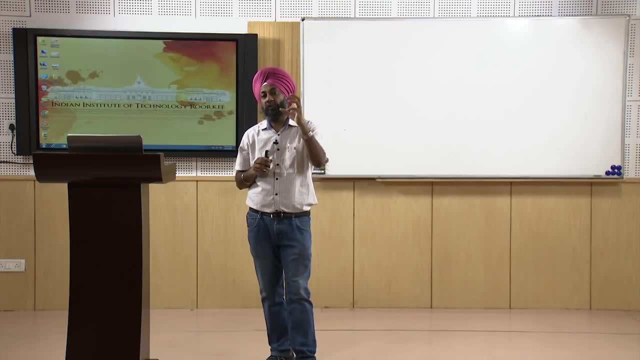 what is the transfer? the transfer is the transfer of the molten plastic from the transfer port through the sprue into the mold cavity. so at least three examples we have taken: injection molding, rotational molding, transfer molding. let us take another example: compression molding, compression. so we are applying the compression force. so the names are coming out from the 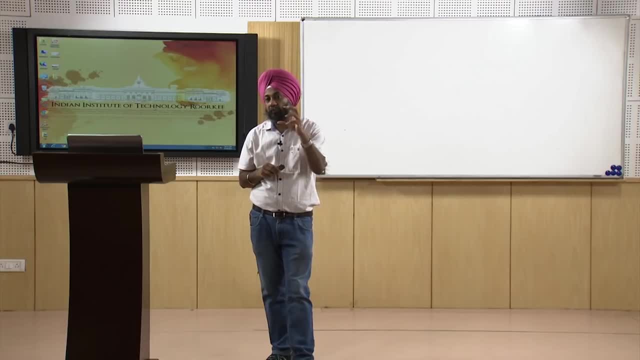 basic mechanism involved in the process of deforming the molten plastic into the desired shape. so here you can see blow molding now. blow molding means we have to blow the air, like usually we blow the air by our mouth. so that is the principle of blowing. so here also the 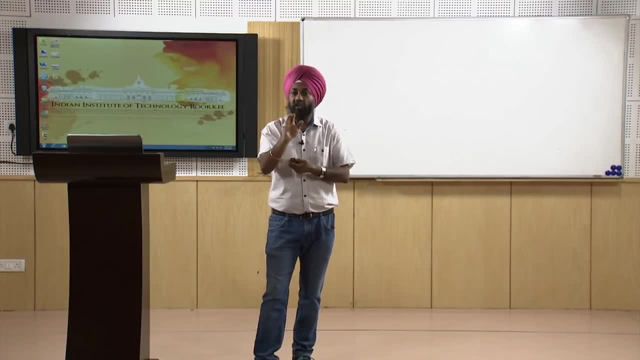 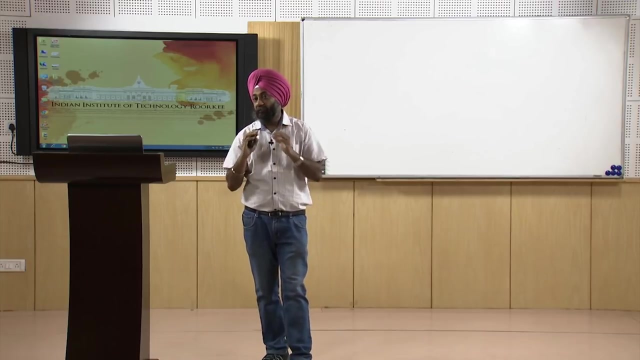 plastic will be deformed by pressurized air and the plastic will be pushed towards the walls of the mold and it will take the shape of the mold. so, whatever we study, whatever we learn, we have to take into account that. why we have to always answer, why we have to. 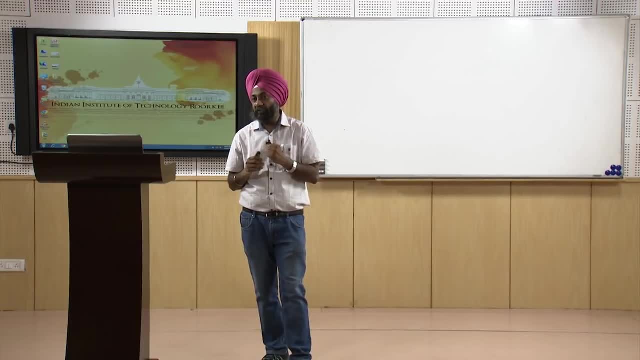 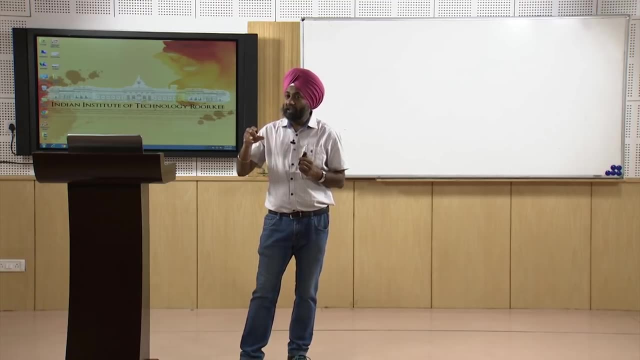 understand that why this name is given. and once we are able to understand, appreciate that why this name is given, we will never forget the process throughout our life. so blow molding means there will be a mold and we have to blow something. now that blowing thing is the air, pressurized air, and that will force the plastic against the walls of 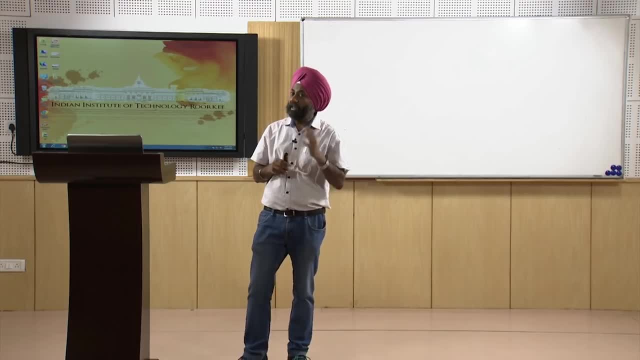 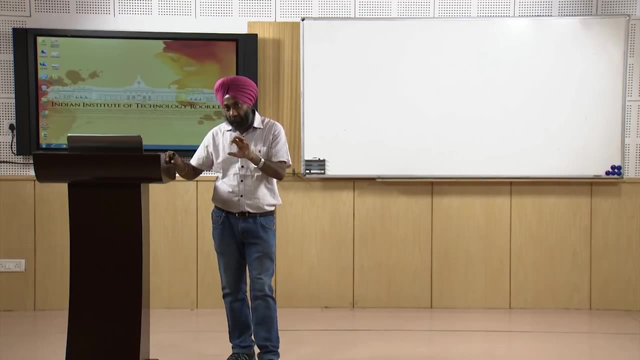 the mold and the plastic will take the shape of the mold, so that ah blow molding procedure we are going to understand today. we are going to understand it with the help of the plastic, of diagrams, we are going to understand it with the help of a animation, so that it becomes. 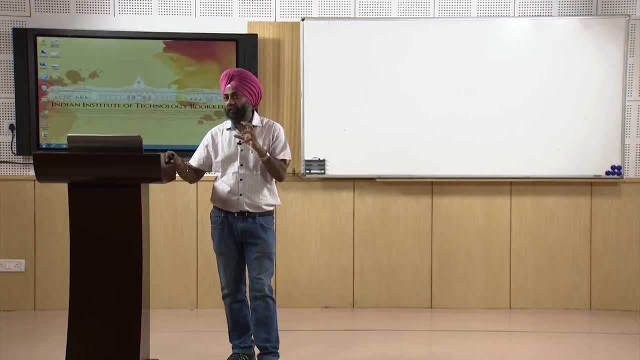 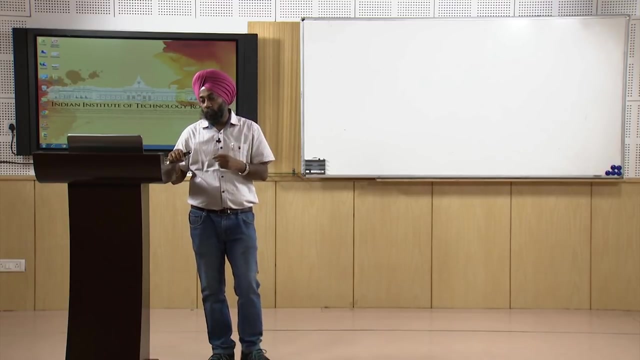 clear in our mind throughout our life. we remember that what is the process of blow molding? even if we see a plastic bottle, we should be able to explain that, how this process has been made. so that is the basic, fundamental, we can say, objective of todays session. that is, blow. 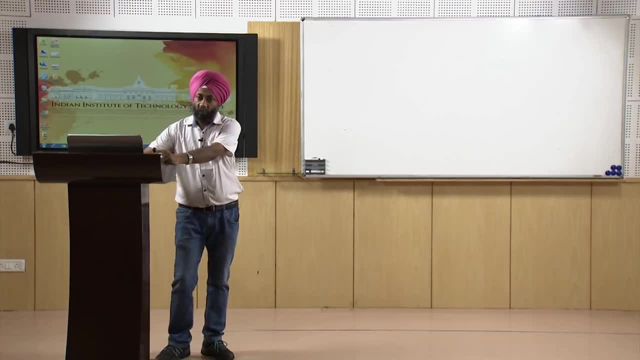 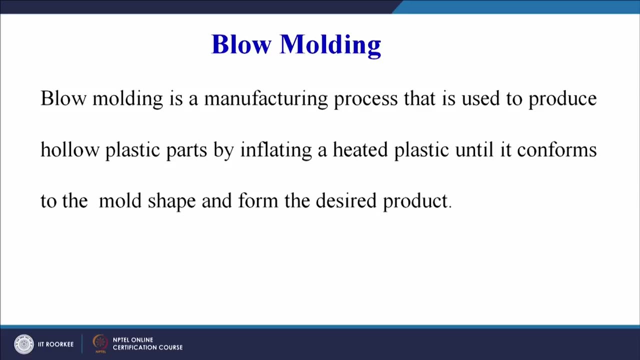 molding session. let us now go step by step. now, what is blow molding? blow molding is a manufacturing process that is used to produce hollow plastic parts. so first thing, we should remember the application, why this process has been developed that is used to produce hollow plastic parts, by how that is done: by inflating a heated plastic. so inflating means. 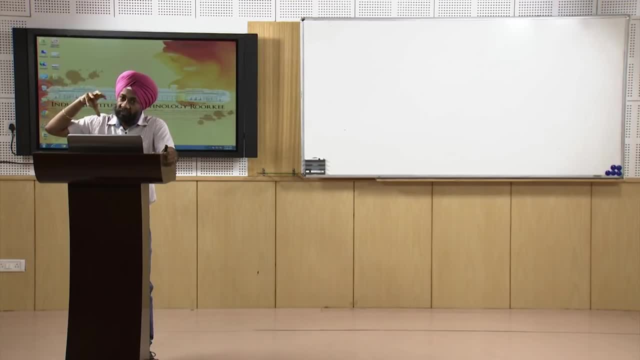 we have to blow, we have to inflate it, we have to inject air inside so that the plastic inflates and takes the shape of the mold until it conforms to the mold shape. so we will apply the air pressure in such a way that the plastic is forced against the 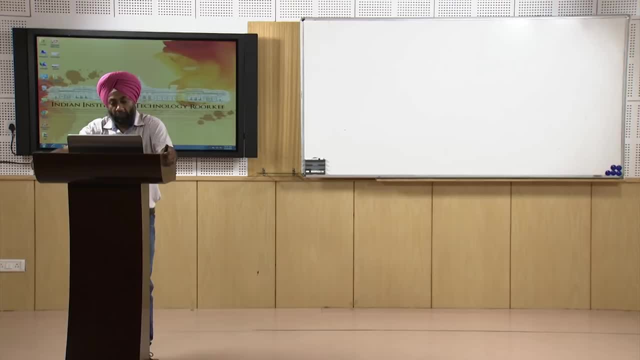 inner walls of the mold and sticks to the inner walls of the mold and then it will form the desired product. so there are three important things. first is a raw plastic material, which usually we called as a parison. then we are injecting pressurized air inside the it is. 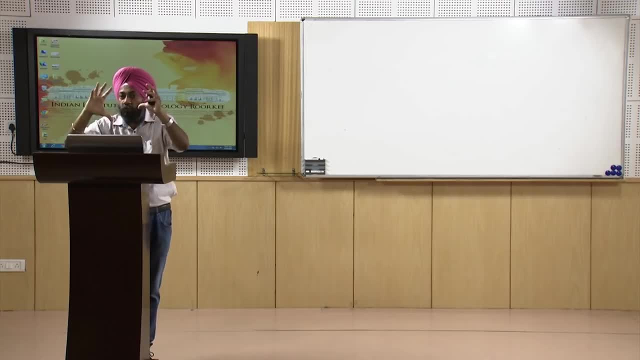 blowing like a balloon and then it adheres outside to control the shape of the plastic so that the plastic gets inflated and it is forced against the inner parts of the mold, and when the mold opens we get our desired product, and before that there is cooling of. 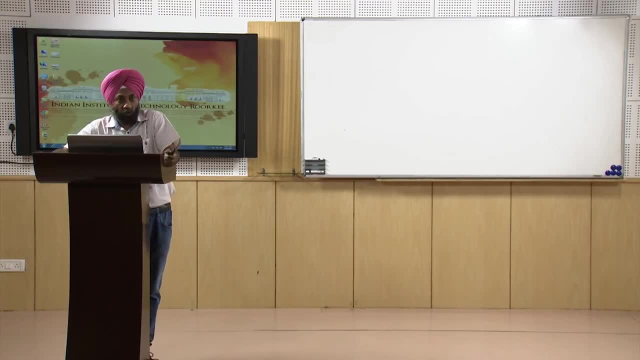 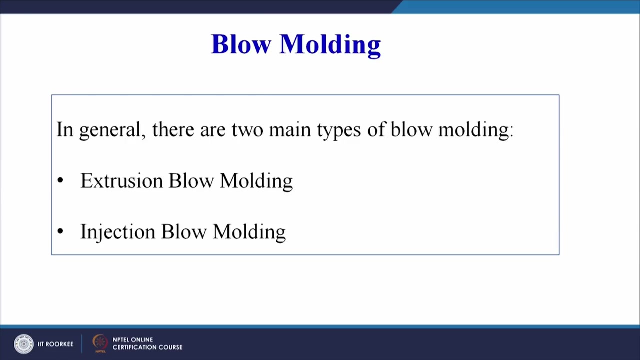 the plastic so that it becomes sufficiently rigid and solid so that it do not deform once the mold has opened. so that is the basic principle of a blow molding process. i think you will be able to appreciate it better when you see the diagram. blow molding process can broadly be classified into two categories. there can 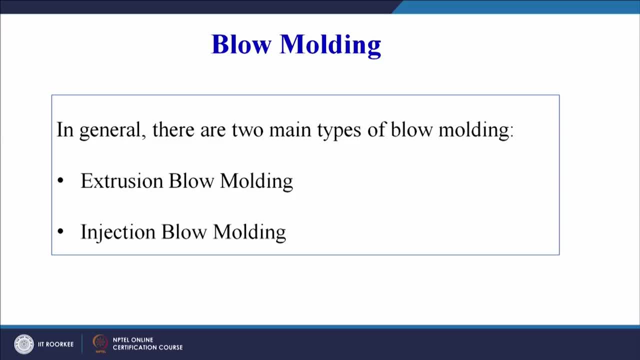 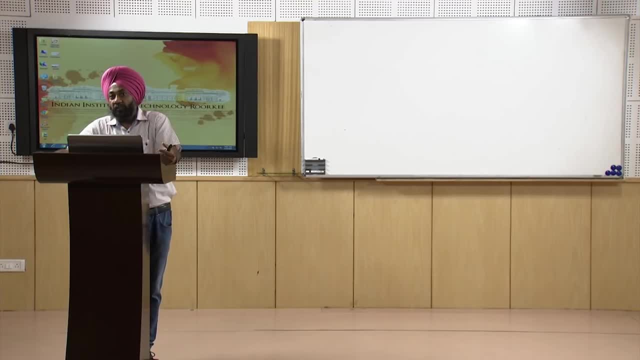 be other classifications also. these. these two classifications are extrusion blow molding and injection blow molding. now, these two classifications are based on that raw material that we use for extrusion process. so the parison, par На and the parison is used as a raw material. 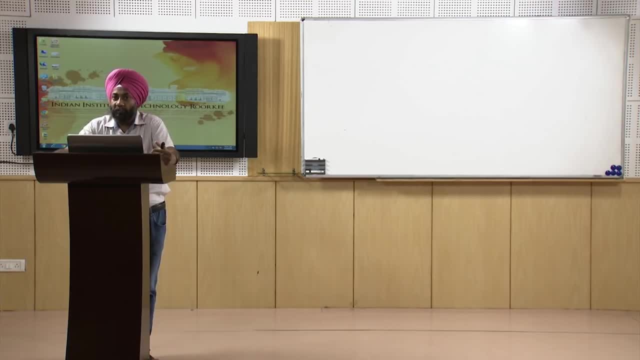 in blow molding and the method for making the parison. if it is extrusion, then we called it. called it as extrusion. blow molding is used in the recovery process, so that it was a crystal cutting procedure with crazy다가 which allows for the order of küçükин, the nutritions have growth in the processes provided enjoy of it and the method for making it an made solid. then we call it with cap enlargang and the method of 안녕. in the second process it interests each material type and which you can theization, check together and test if you. 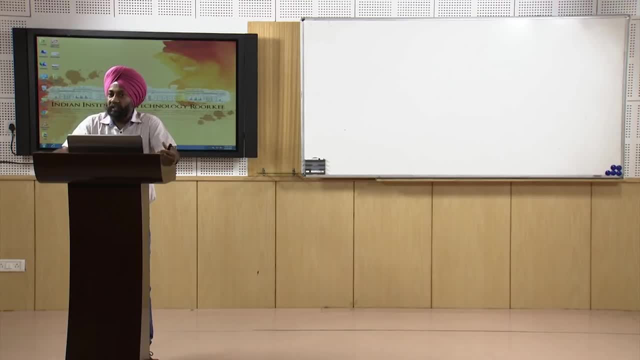 fabrication or processing of parison is injection molding. in that case we will call the blow molding process which uses a parison made by injection molding process as the injection blow molding process. so there are combination of two processes. now most simplistic diagram is given a schematic on your screen so you can see initially. this is the shape that the 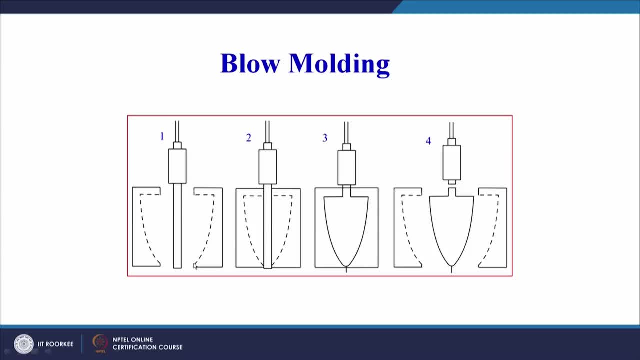 dotted portion is the inner part of the mold and this is the shape that we want to make this inner portion and this is a split mold. this is one half of the mold and this is another half of the mold. through this pipe we will have pressurized air that will come inside. 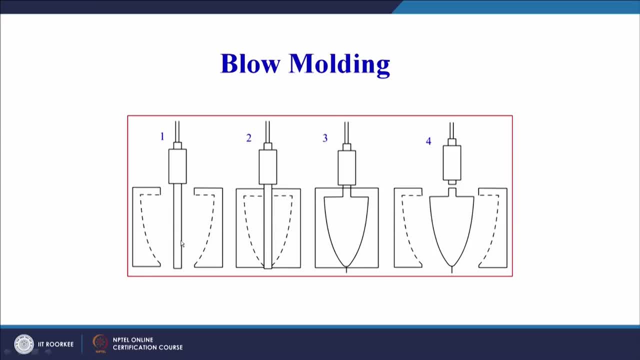 and this is the parison or the raw material that can be made by extrusion process also. this can be made by injection process also. so this parison is hollow and it is open from here. so in the ah the air can be pressurized through this particular nozzle into this. 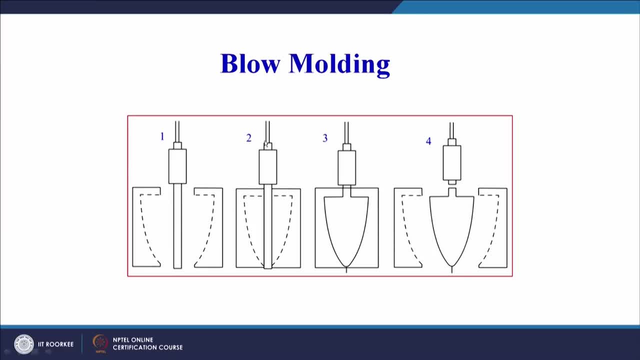 parison and the parison will blow. so the second stage is we can have pressurized air. the mold has closed in this case. here you see, the mold is open. second stage: mold has closed down and we get our final cavity or the final replica of the product that we want. 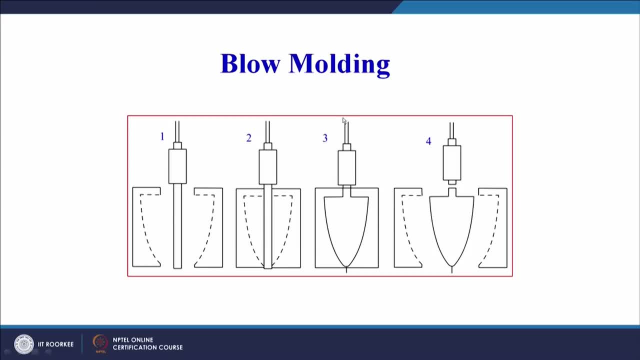 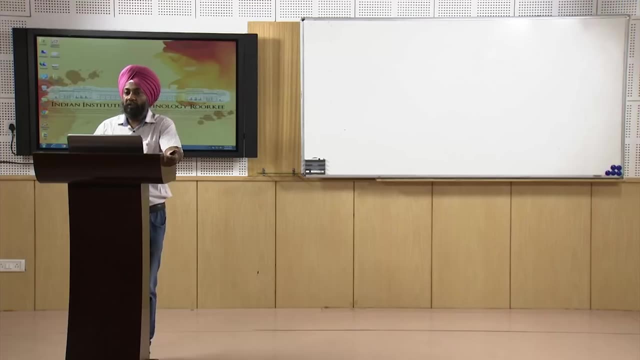 to make. so this is a hollow cavity. third, air pressure from top- the parison you can see here- blows and takes the shape of the cavity inside the mold and finally the mold opens and the product is taken out. so this is our final product. so we can see, pressurized air is used in this case and if you remember and if you have attended, 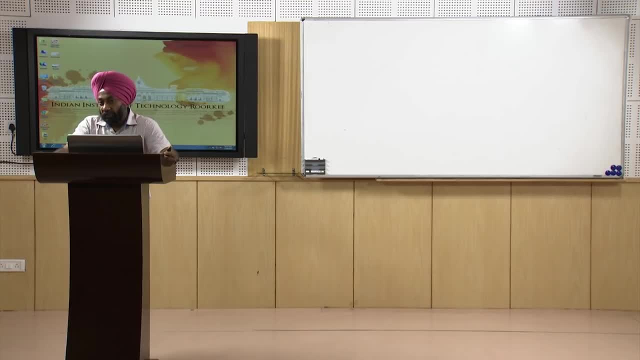 or ah heard to the discussion. in the case of extrusion process. there was a blown film extrusion process in which there was again this pressurized air was used in order to blow the plastic and then finally there was a ah- you can say- breaker in which the two films got collected. so that was similar type here. 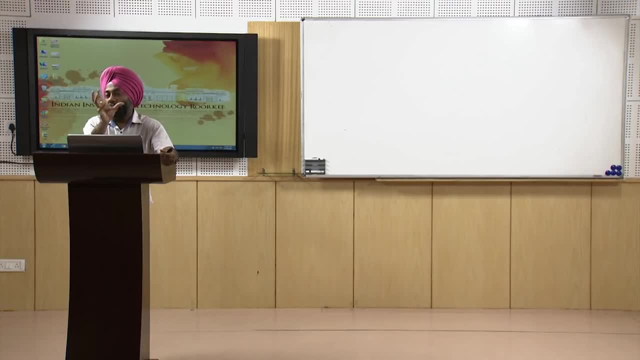 also pressurized air is used. but here we are making a hollow product there after going we there were breakers, so the two films were again combined together and we were able to make a film. so it was a blown film extrusion process. so there also pressurized air was. 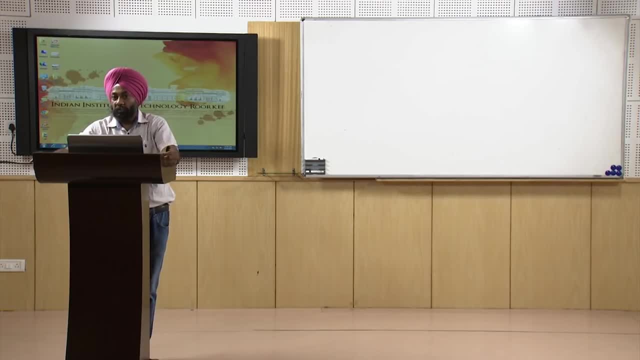 used. so here again, pressurized air is used but to blow the parison as per the desired shape of the product. This is the working principle of the blow molding process. so here you can see. ah, another diagram 3d, which is much more explanatory as compared to the previous one. the source: 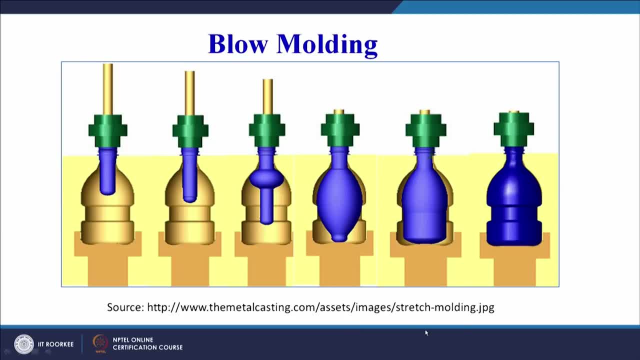 is given the metal casting dot com on your screen: stretch there. name the process as stretch molding. so i think the basic principle remains same. this blue color is the raw material. this is called parison and through this section We will have our pressurized air. so this is, ah, the first stage. the second stage, it is 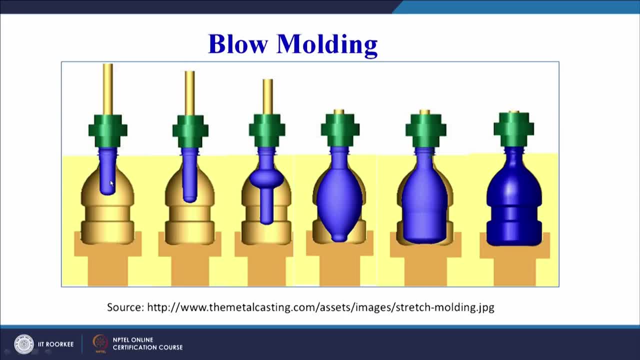 it has started to blow. you can see the size difference between this and this. and finally, when the air pressure is maintained, it further blows. next stage, next stage and the final stage, it finally takes the shape of the bottle. so this is the blow mold basic principle of 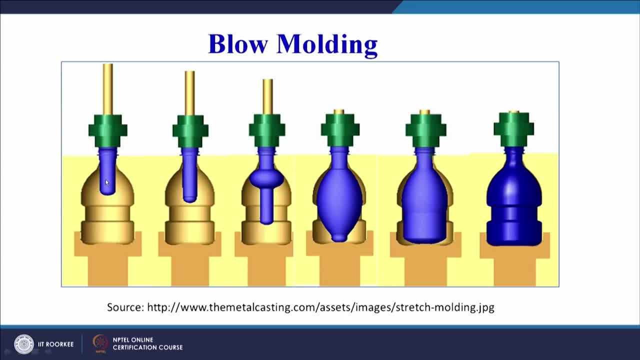 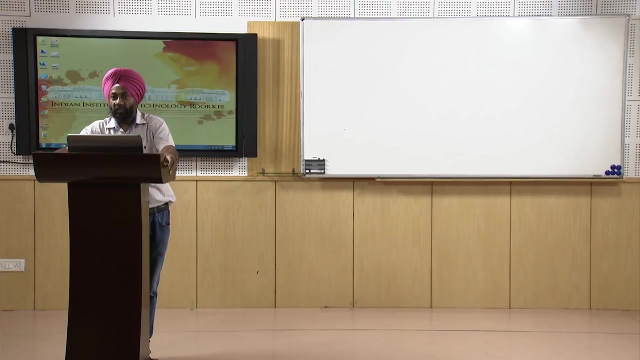 blow molding. The blow mold pieces are not close. it is the form of the plastic mottled. that is where the air goes in the mold. so there is a parison raw material which is there inside the mold. pressurized air is supplied from the top and 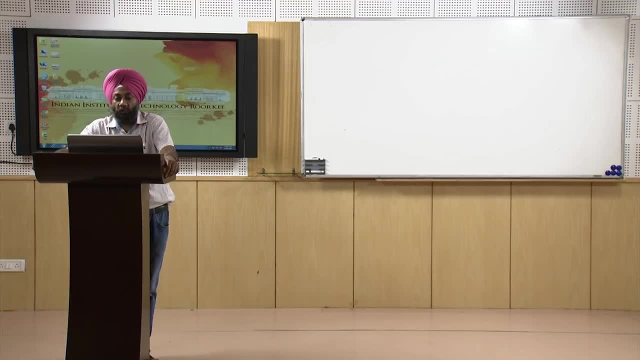 then it gets inflated in sequential or step wise manner and finally takes the shape of the final product. Now, whatever i think we have understood from these diagrams, let us read all these points to just strengthen our understanding the and forming it into a parison or a preform, so that blue color raw material, that is basically 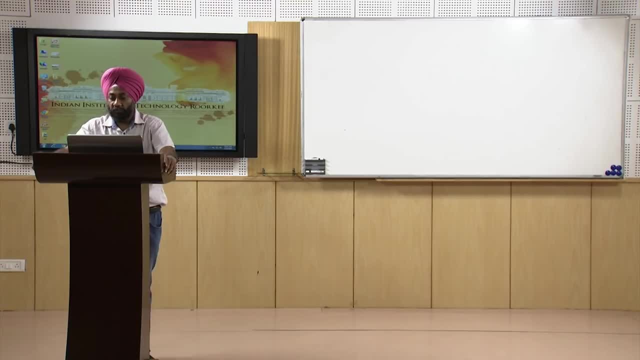 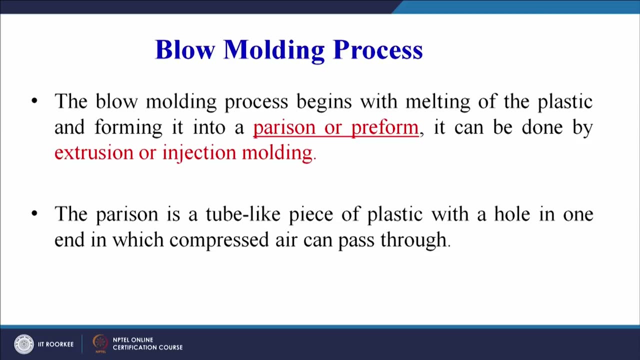 parison, so it can be made by extrusion or the injection molding process. it can be done by extrusion or injection molding. that is the first stage. the parison is a tube like piece of plastic with a hole in one end in which compressed air can pass through, so it 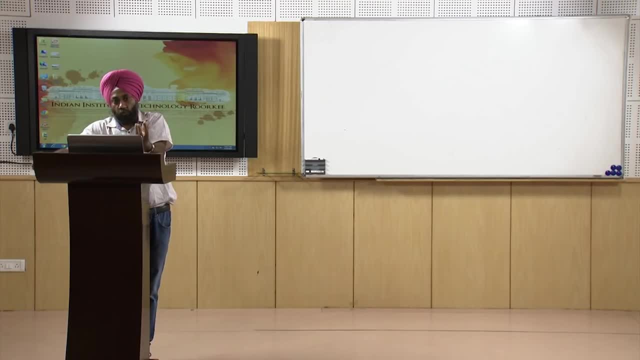 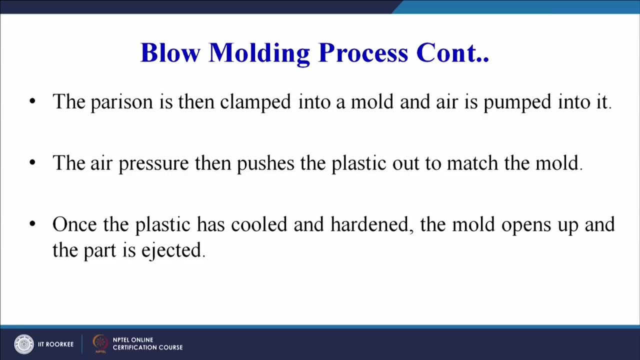 has to be: ah, a open from one side and closed from the other side. the opening side will allow the air to pass through. the parison is then clamped into the mold and air is pumped into it. the air pressure then pushes the plastic out to match the mold. so i have already explained. 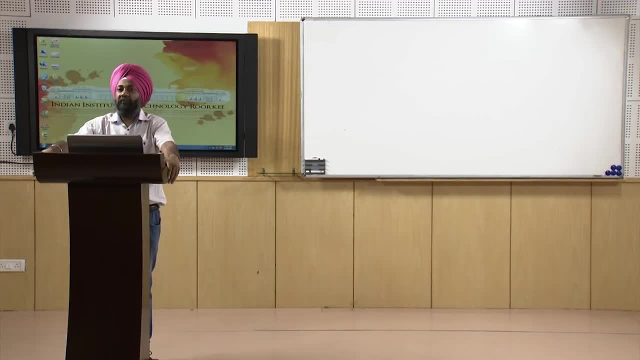 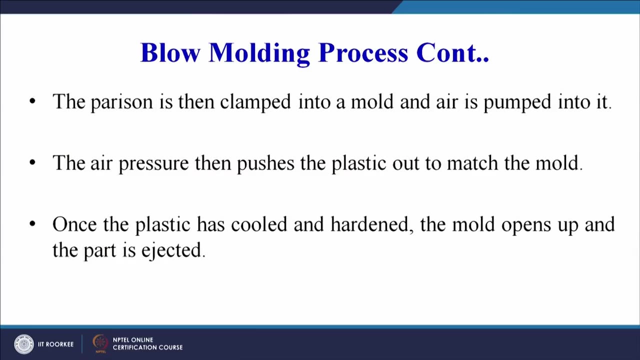 when it will inflate it will go to the inner cavities of the mold, so it will adhere to the inner shape of the mold. once the plastic has cooled and hardened, the mold opens up and the part is ejected. so this is the first stage of the parison. so the parison is then clamped into the mold. 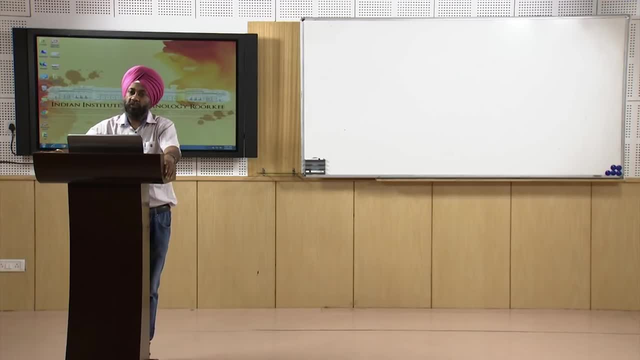 this is, as i have told you again, a split mold type of process. so once the mold will, once the product has solidified- that has to be decided earlier that- we will see in the process parameters that we can control in this process. so once the product has solidified the mold, 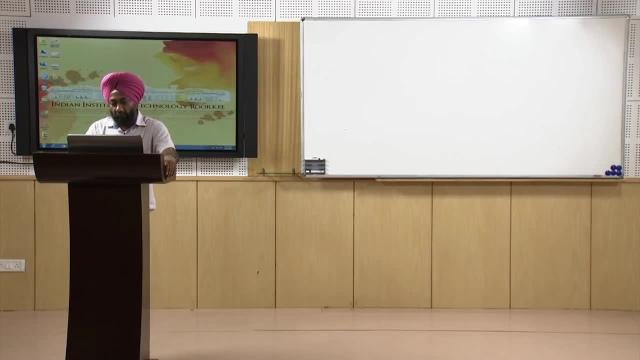 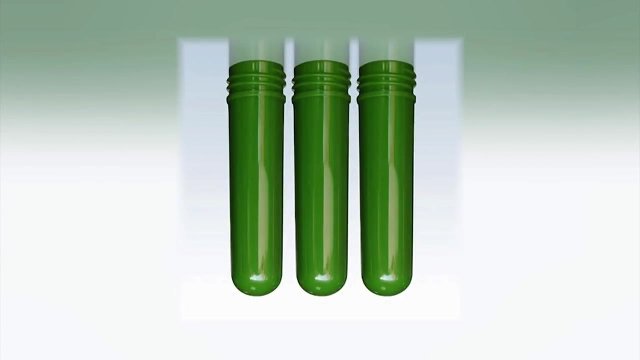 will open and our product would be released. let us try to understand the whole process with the help of a simulation. the steps will be same, whatever we have already discussed. so this is the material which is generally used: polyethylene tetra plate. so this is. these are the parison, the raw material that will 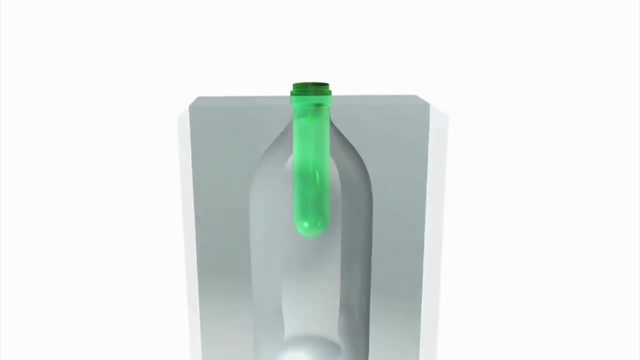 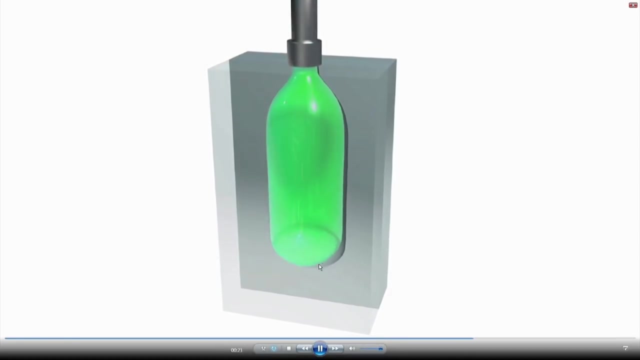 be used to deform. this is, you can see, the mold is already closed. this is a parison. air is coming from top and it is inflating the raw material, the, it is adhering to the shape of the mold and finally, the mold will open and the mold will be closed. so, once the mold 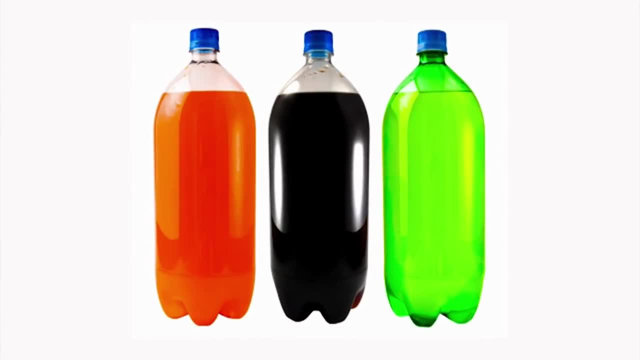 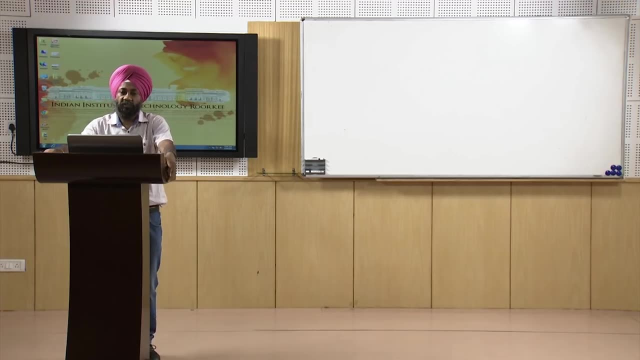 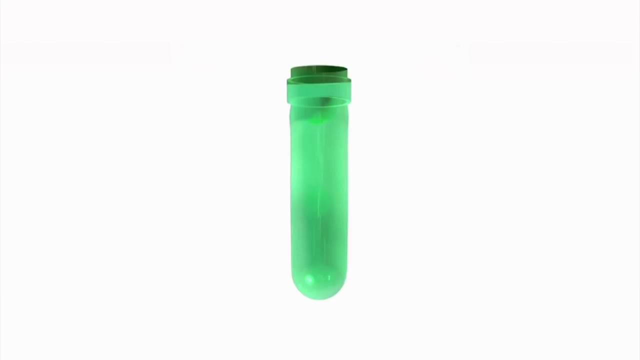 is closed, then the mold will open and the mold will close, and the mold will close and open and take the final shape. so there you can see. ah, most simplistic representation: polyethylene tetraphlate. once again you can see the simulation. there are number of such simulations available on youtube so you can refer to them for better. 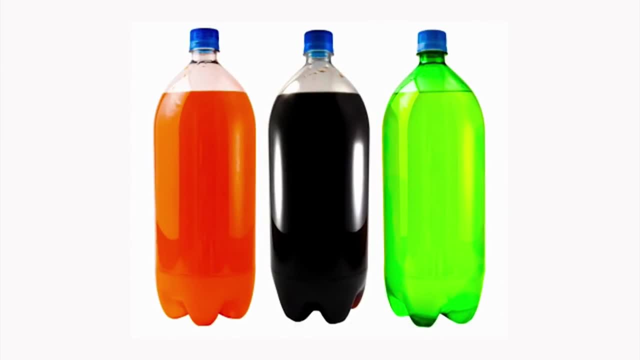 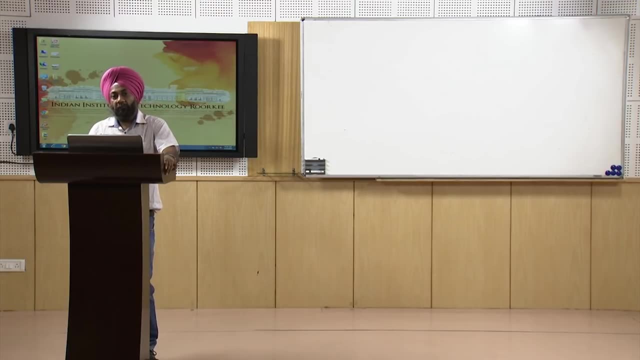 understanding and all the steps may be mentioned there, that is, from mold closing. mold closing to the fixing up of. the first will be the fixing up of the parison at the desired position, then closing of the mold, then starting of air pressure and then inflation or maybe blowing. 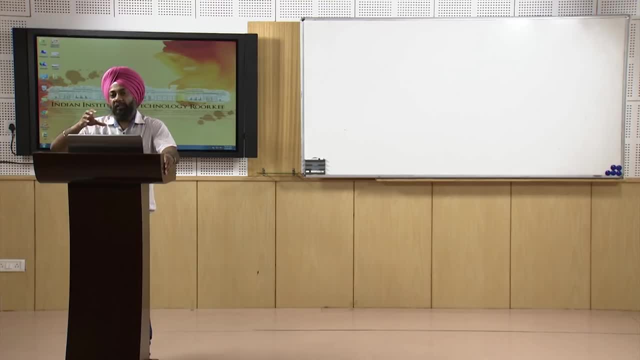 of the parison, sticking of the parison, or maybe the parison then takes the shape of the mold cooling process: opening of the mold and ejection of the final product. so this is showing maybe the most important part, that is, the blowing of the parison and the ah molten sorry, the plastic. 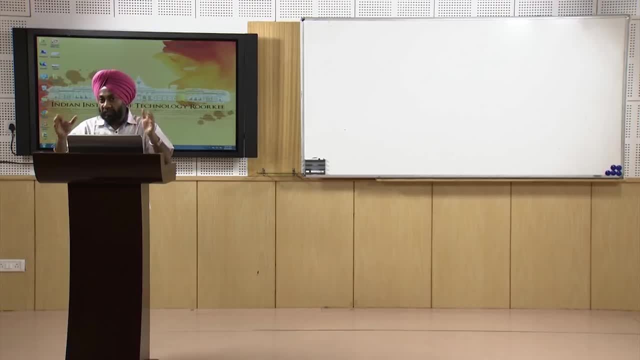 taking the shape of the ah mold. but there are other steps also after all, afterwards also and prior to the ah blowing process also. so you can see other videos which will give you even better representation of the blow molding process. now, what are the parameters that need to be controlled in this process? you can see: 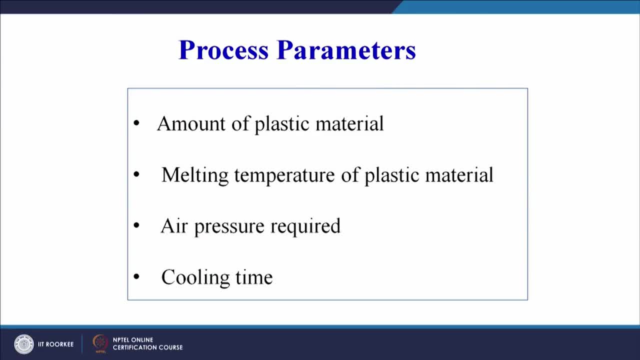 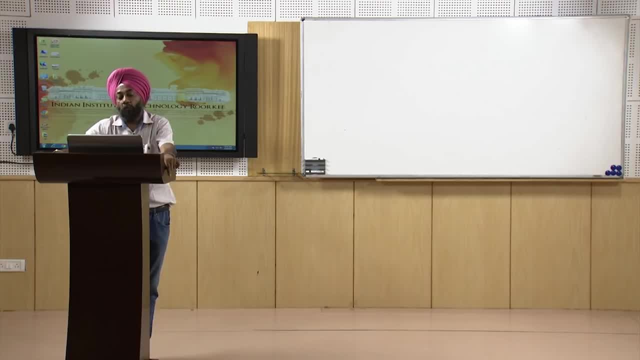 ah, both vocal, ah wh인 the, the that needs to be controlled. Ah then, ah, that needs to be controlled. if that needs to be controlled, of course you can get to it. counseling process will disめal chaoticidet墨 realize, as well as other stuff, the one relationship in to this process, including the processes to build, orå, serious to build, amplify the non��, the amount of plastic materials that we will need to can control that. what type of Paris? and should be made the melting temperature of the plastic material. so these two are important from the manufacturing of Paris and points out of you, because that Paris and it is carry, it is ready. then we will have to just blow. 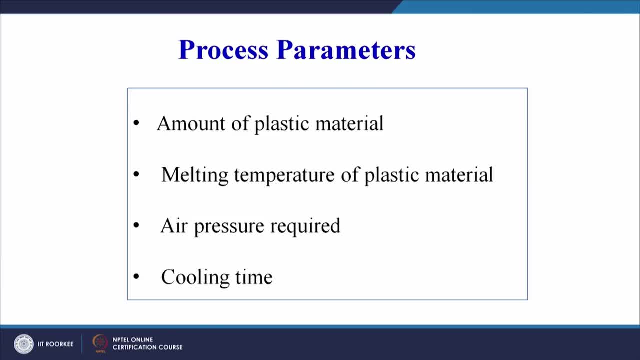 it and it will take the shape of the mold. air pressure required definitely during the blow molding process. we have to see very high air pressure may lead to certain defects in the blow molded part and very low air pressure may leave the mold unfilled and the parison. 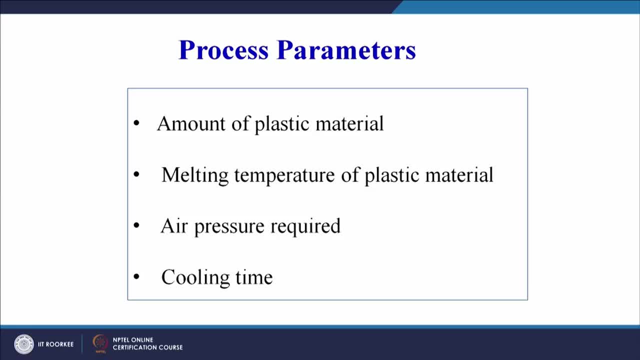 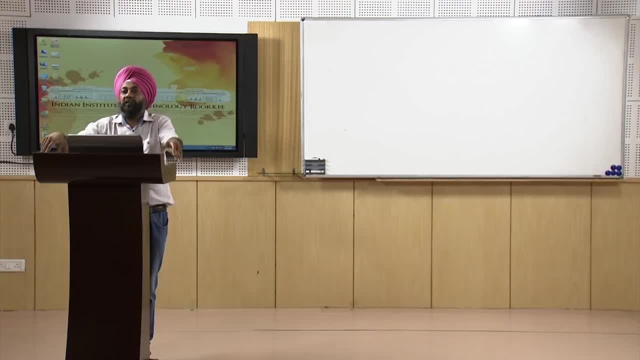 may not take the exact shape of the mold, so the pressure has to be optimal. and then, as i was just discussing, the cooling time, the period for which the two halves of the mold will remain closed. that has to be judiciously selected, because once the mold opens and the 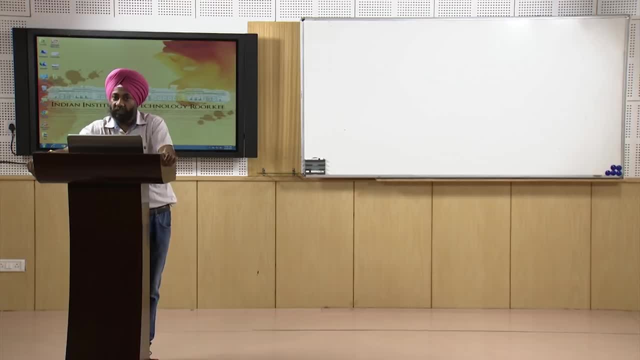 product is taken out from the mold, it should be sufficiently rigid and it should be sufficiently, we can say, solidified so that it do not deform after coming out from the mold. so we have to ensure that during the cooling period, the two halves of the mold remains closed and 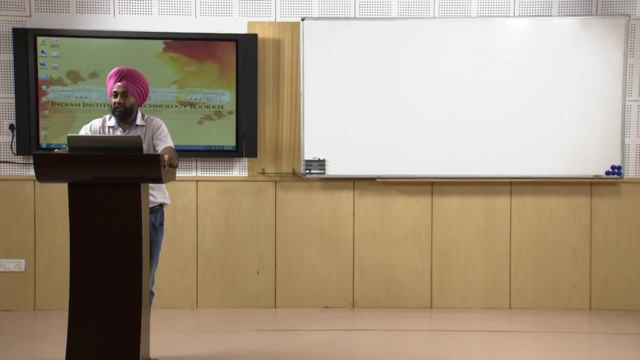 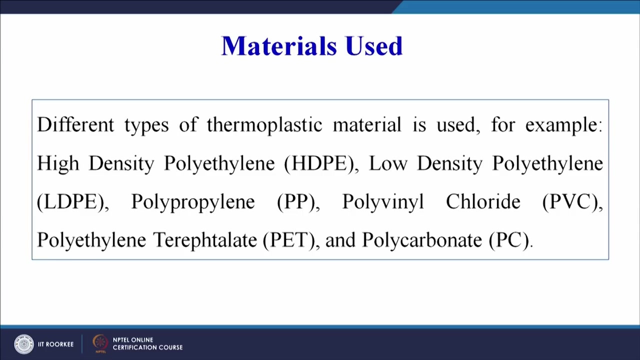 the product becomes ah product becomes sufficiently hard and sufficiently cooled. so that has to be taken into account. now, what are the materials used? one is the most common bottle, plastic bottles that we use: mineral water, soft drink plastic bottles. though that is already. you have seen polyethylene tetraphlate pet bottles, then this can process. 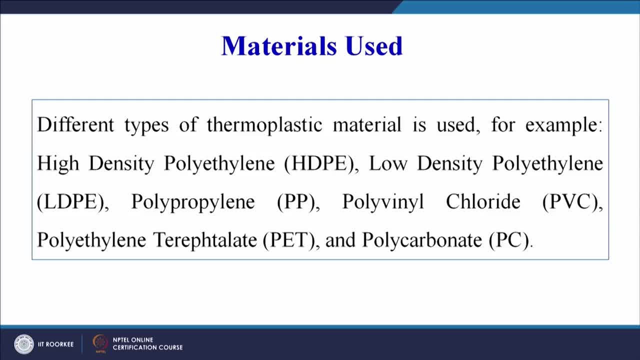 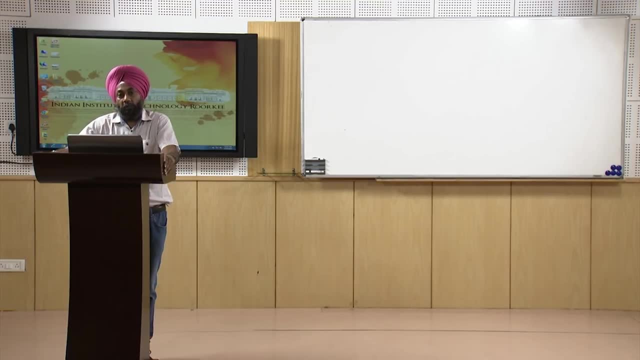 can also be used as a for hdp. high density polyethylene can be used for low density polyethylene, probably propylene, polyvinyl chloride, polycarbonate. so different types of materials can be used, as we have seen from the literature. now, what can be the advantages of this blow? 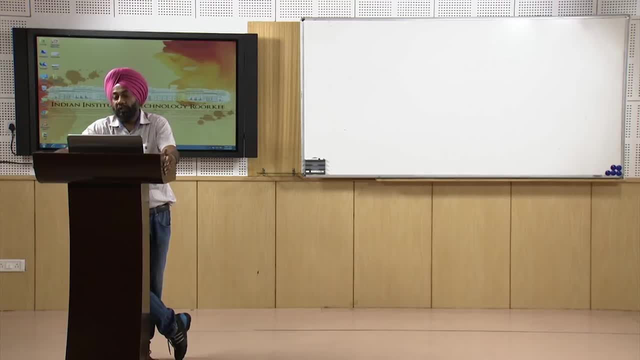 molding process. as you have seen, it can be completely automatic process. so once it is automatic, with no manual intervention, so the fast production rates can be achieved, so you can make hundreds of bottle per hour. so that is that kind of flexibility can be there. so maybe, ah, different types of machines are there. 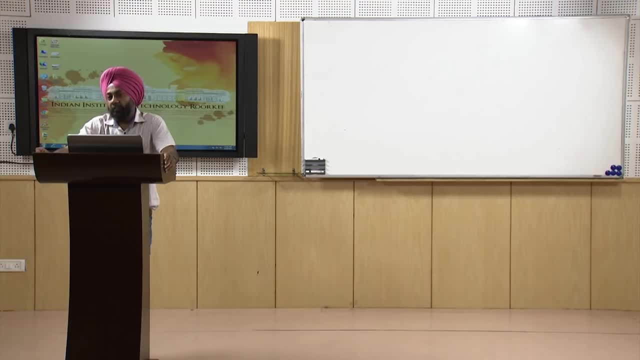 blow molding machines are there with different process capabilities, but the production rates are extremely, extremely fast in case of blow molding, as we have seen in rotational molding- the hollow plastic parts that are made by rotational molding we have seen- the process cycle is maybe extended, so a lot of time is taken to make a product by rotational molding. 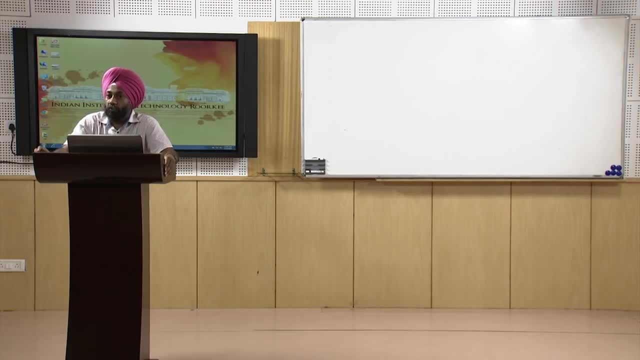 process. but in blow molding process that problem is not there. it is a very, very, very, very fast process and the tooling cost is also not that high. then you have seen in one of the diagrams that at very ah, typical geometry of a bottle can be very easily made by blow molding process. so the above, it has the process has the ability. 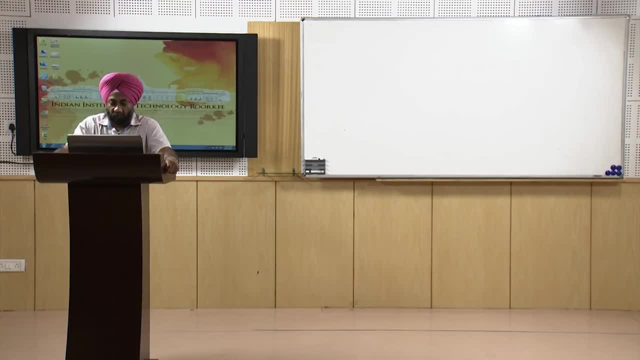 to mold the complex parts or the complex products. scrap generated is minimum. as you can see, the parison is pre predefined, as we have already seen in the process parameters that we have to decide on the amount of raw material, we have to decide on the melting temperature. 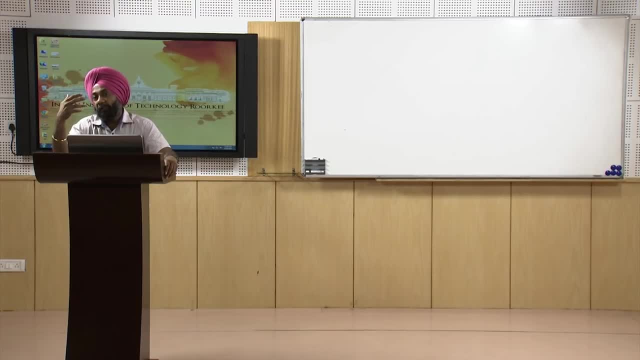 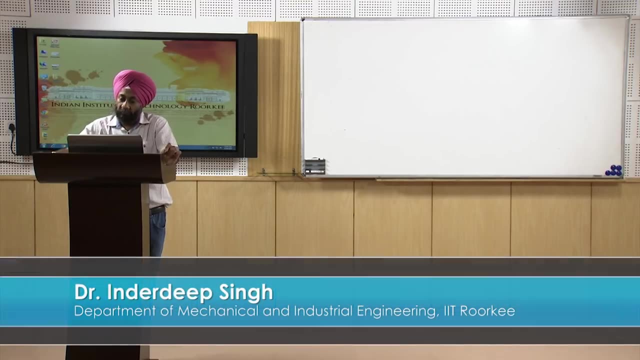 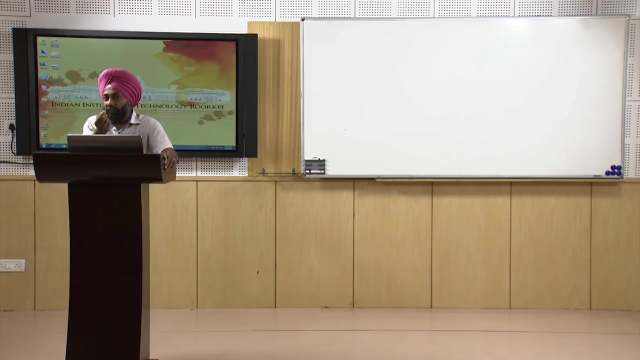 of the raw material. so we take decision, prior to bringing the raw material to the blow molding process, that what should be the thickness ah, thickness of the ah parison, so all those parameters are controlled. so therefore there is little wastage of the raw material. only from the bottom side, whatever is clamped between the mold that may have to be removed, that is. 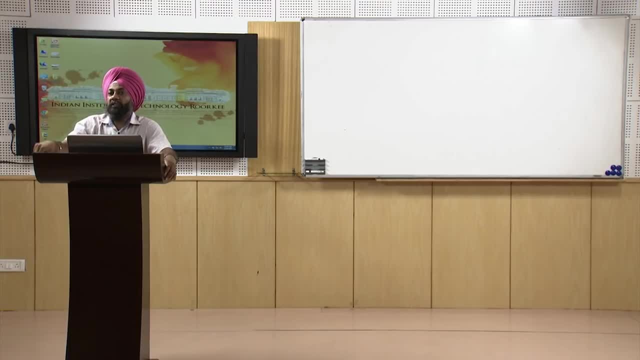 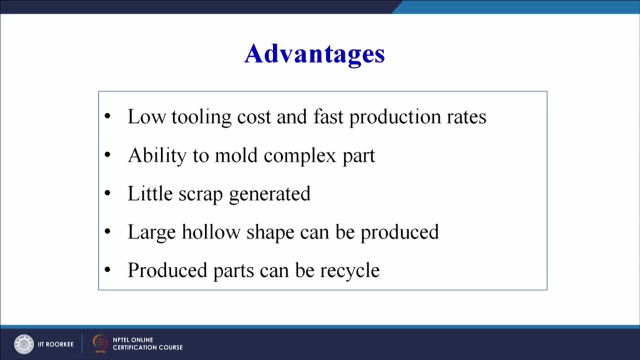 one thing, and from the top also. a little bit of material scrap is produced, so the ah little scrap generated, so minimum wastage of raw material. large hollow shapes can be produced, but not as large as we can produce in rotational molding. produced parts can be recycled. so 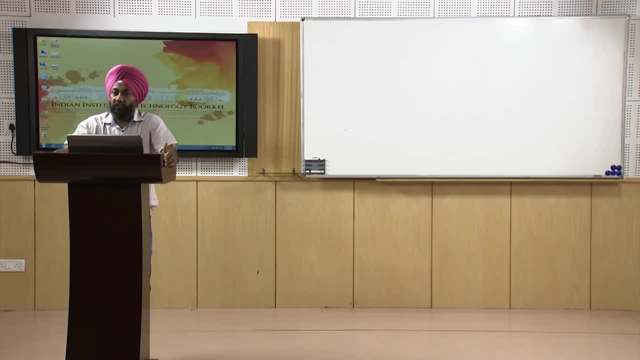 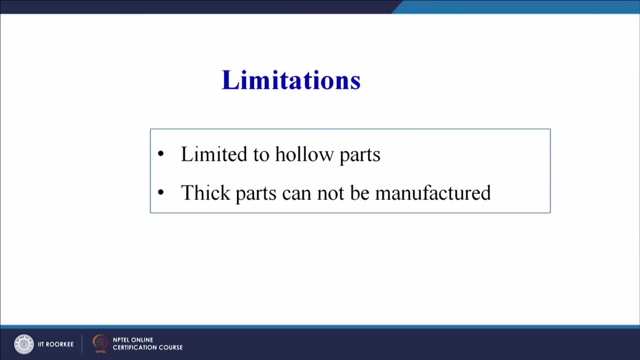 that is, that facility is also available and mostly is used for making thermoplastic parts. what are the limitations of the process? now, limitations: this process is only limited to hollow parts. thick parts cannot be manufactured. ah, So it is the thickness of the wall of the product that we are making. if you see the 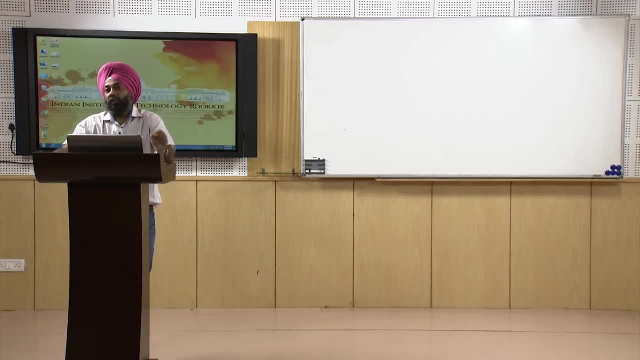 plastic soft drink bottles, the mineral bottle. so the thickness of the part is not very large. so the ah sheet thickness, that is that we achieve, or that is not very thick in case of the blow molding part. so that is one ah limitation and the another is that we can. 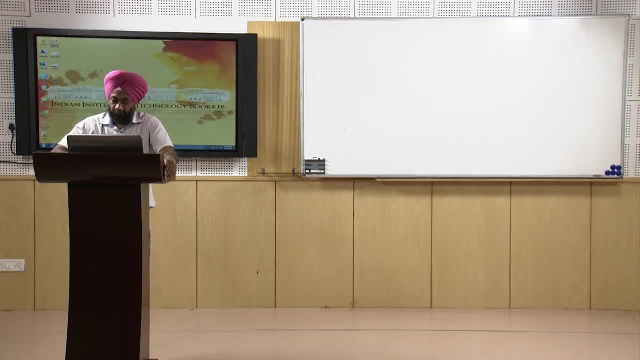 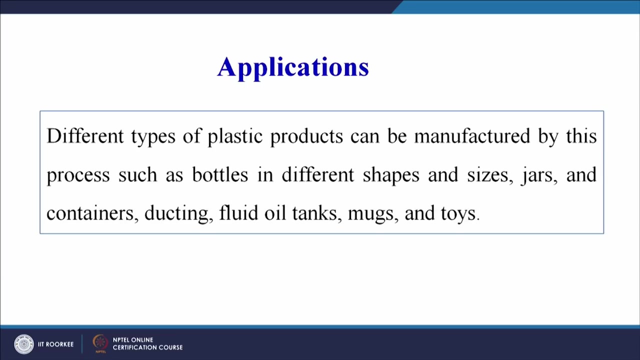 only make hollow parts using the process. ah, ah, ah. one of the application is absolutely clear to all of you. as we have seen in the diagrams also, the simulation also, or the animation, different types of plastic parts can be manufactured by this process, such as bottles in different shapes and sizes, as we have seen. you may be. seeing number of plastic bottles for different products are coming: small size, large size, different ah geometries, and then there may be a place for a grouping mechanism also, so different shape sizes can be produce. ah can be produced. ah we have to design is the mold. so the plastic will take the shape of the mold. so whatever, 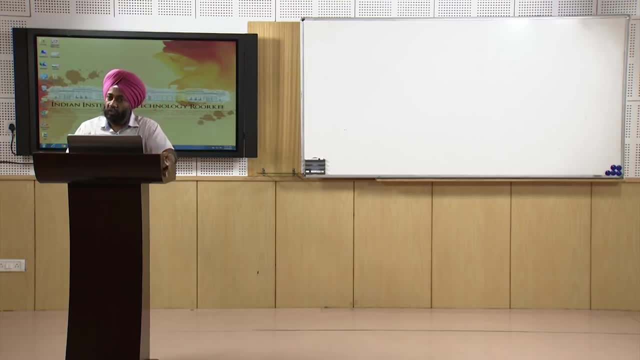 mold. we design accordingly the shape we can produce. so that is the that is the beauty of the process: that we can produce different shapes using blow molding process. jars can be made, containers can be made, ducting fluid oil tanks, mugs and toys. so there are, you can. 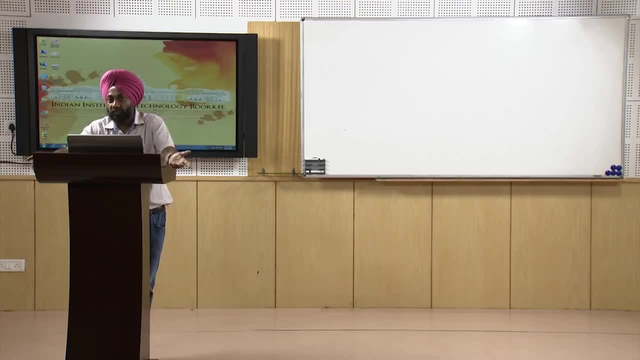 see there are number of engineering applications, non engineering, domestic household applications that can, or the products that can, be made by the blow molding process. so i think with this we have ah understood the whole process of blow molding. we have seen that, which is the most commonly used plastic that is used for making of plastic bottles in the simulation. 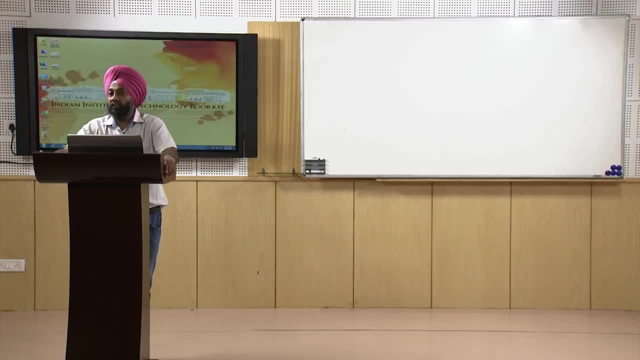 or the animation. we have tried to understand that and we have understood that. what are the advantages and limitations of the blow molding process? so with this we come to the end of our discussion on blow molding. just to summarize what we have covered- because this is our course- is divided into two broad 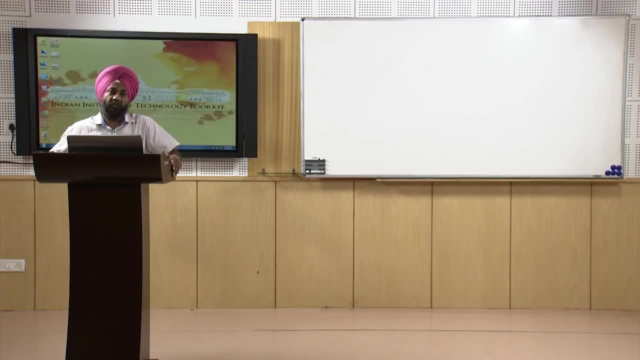 areas. one is the processing of polymers or plastics, and another one is processing of polymer based composites. from our next session we will start our discussion on polymer based composites. so today i will just have a glimpse of what we have covered in polymer. ah, polymer. 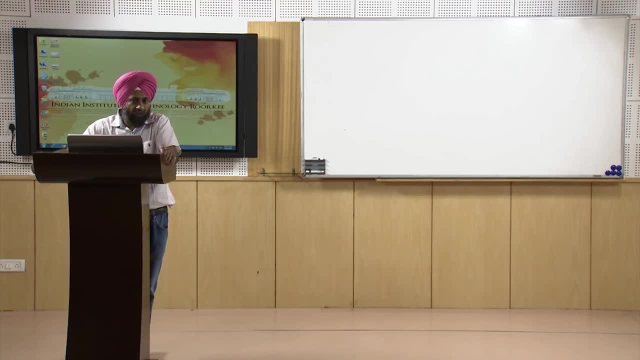 processing techniques and, if you remember, in the very beginning we have had little bit of discussion on the classic process of blow molding process and that is what we have covered. so we have classification of plastics and what are the plastic, what is a monomer and how, what are? 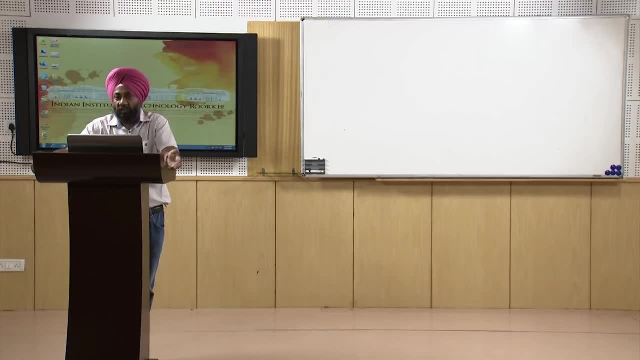 the different types of monomers and how they polymerize to make a plastic. so all that we have covered in the very beginning. but from processing point of view, as our courses on processing of polymers and polymer composites, on your screen you can see the processes that 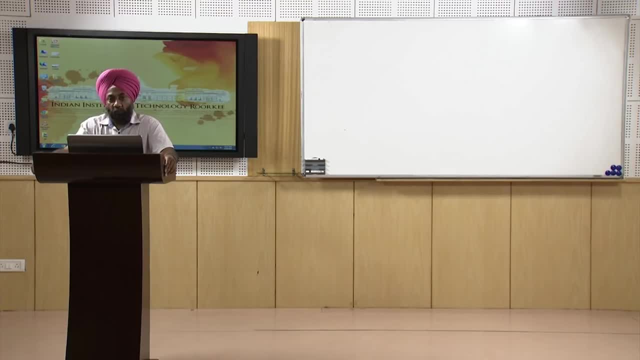 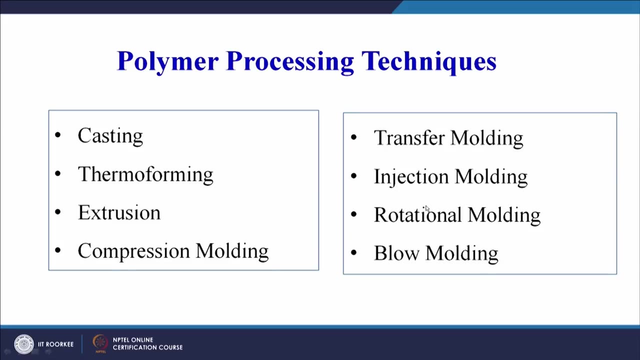 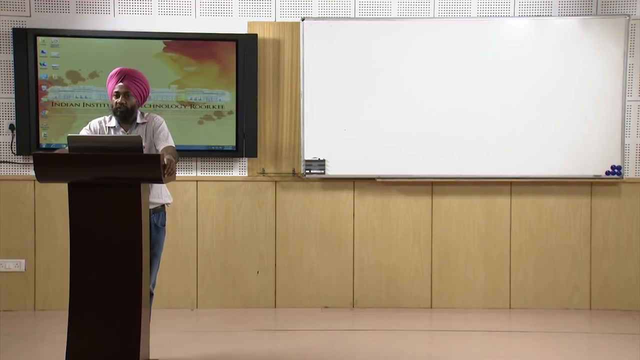 we have already covered. we have covered casting, thermoforming, extrusion, compression molding, transfer molding, injection molding, rotational molding and blow molding. so at least eight different types of processes have been covered for the processing of polymers and, if may be the learners pay attention to what has been covered- at least some fundamental knowledge. 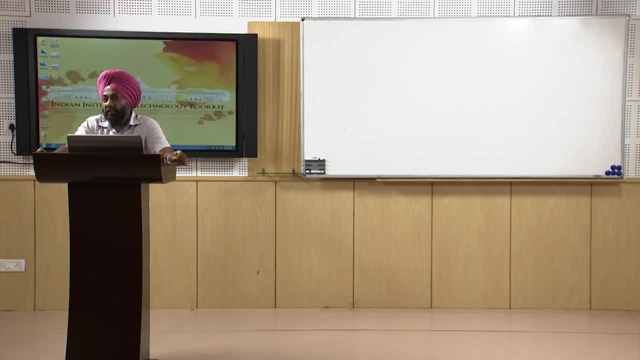 related to plastics has been developed, specifically related to the processing of plastics, and i would advise that, if possible, you can look around and see the different plastic products and try to relate the that this product may have been made by this process, maybe by injection, molding or by compression. 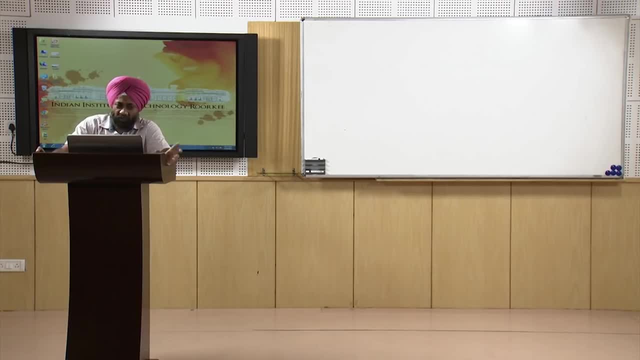 molding or by ah transfer molding. so you can just have a look and i believe that if you know the fundamental working mechanism and the applications of a particular process, you should be, you must be, and you will be able to identify that this plastic product must have been made by this particular process. so with this,